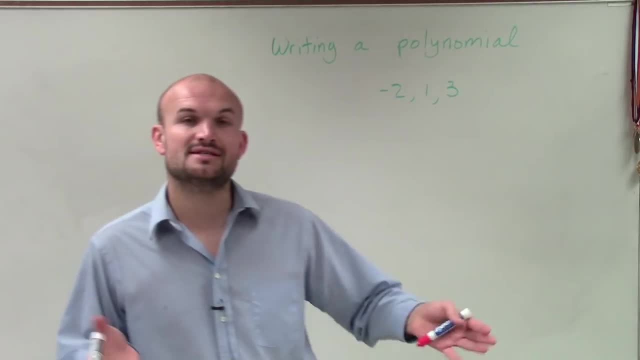 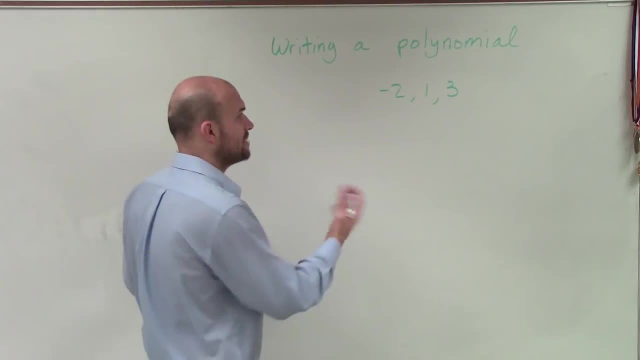 function, So to write it. what I like to do is, you know, we've worked on some problems on giving a polynomial function and then finding the zeros, And one of the methods we used for that was reverse factoring. And so what I'm going to kind of do- to write our polynomial- is we're going to 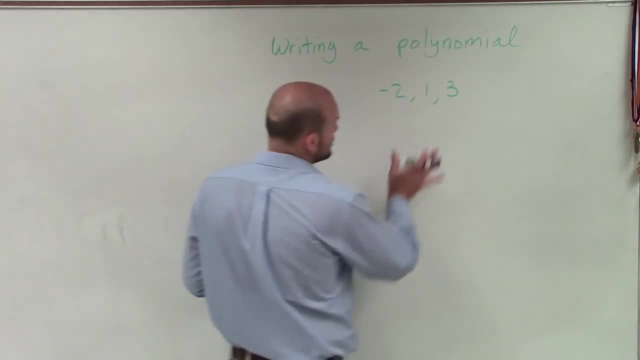 kind of call a reverse factoring technique. So what I'm going to do is, if these each are zeros, I know that we could write them as x equals negative, two, x equals one and x equals three. right, When we solve the problem, we said, hey, here's the zeros. Our final answer would look: 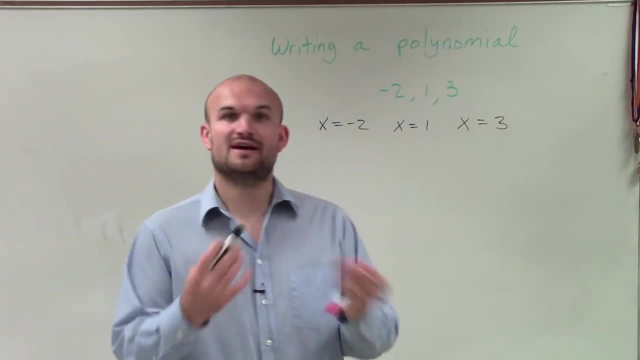 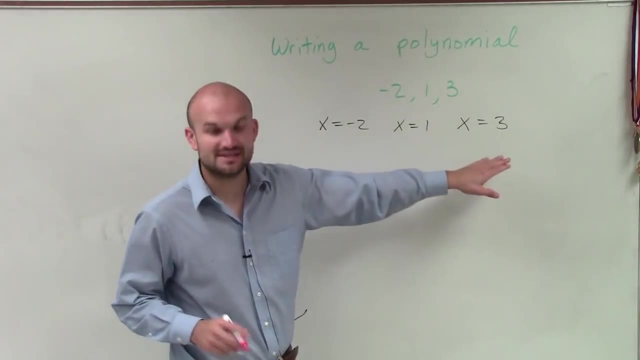 like something like this, because we'd have to go ahead and solve for x. However, we're not trying to find the zeros. We already know the zeros. We're not trying to find the polynomial, So ah. so what we're going to have to do is now, when we write them as zeros. now, what we're going to want. 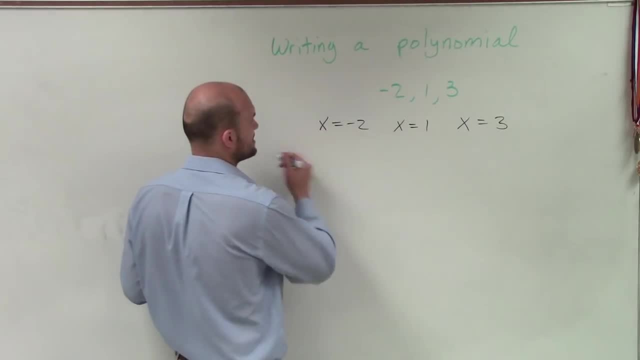 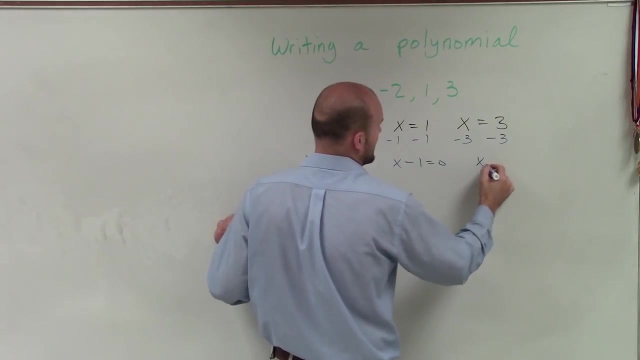 to do is rewrite them as factors. So, to rewrite them as factors, what I'll do is I'll add two and I'll set them back all equal to zero. So I'll have x plus two equals zero, x minus one equals zero, and x minus three equals zero. Now, why would I set them all equal to zero? Well, 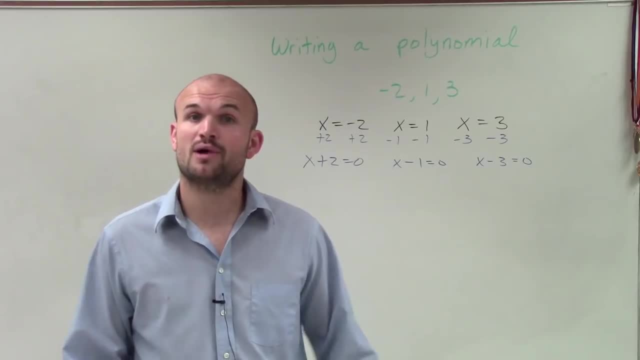 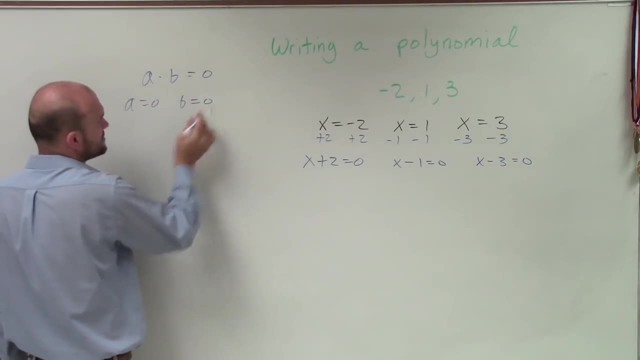 remember how we got them to equal zero, but was by applying the zero product property right. When we had a zero product, we had a zero product and we had a zero product and we had a zero product because we'd already have a times. b equals zero. We say a equals zero and b equals zero, and then 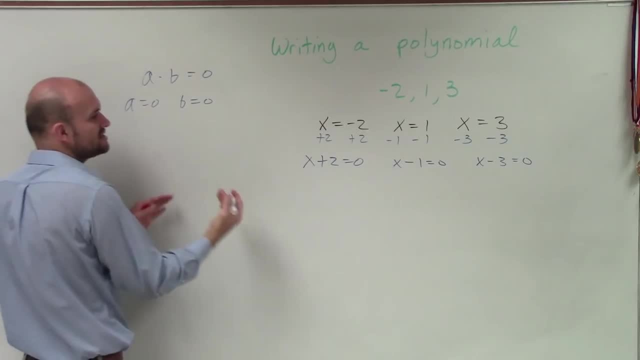 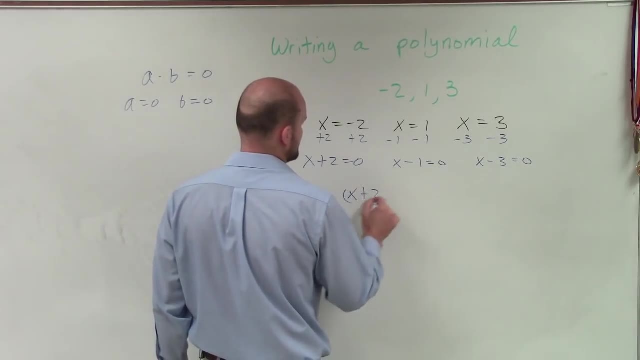 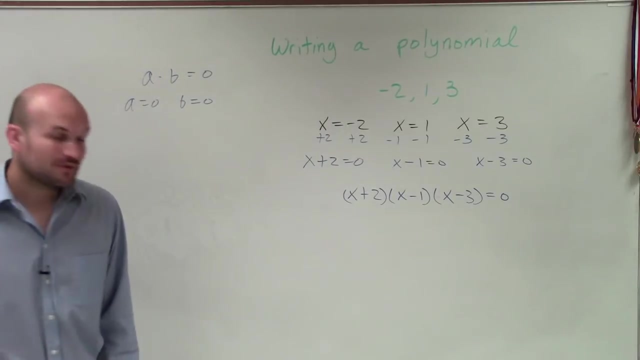 we can solve. Well, we already have this point. Now we need to write them. since they're factors, we can write them as a product of each other, all equal to zero. So we can say: x plus two times x minus one times x minus three equals zero. Now we're going to have a little fun. 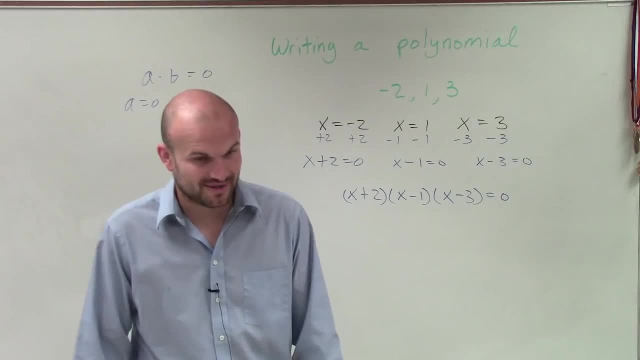 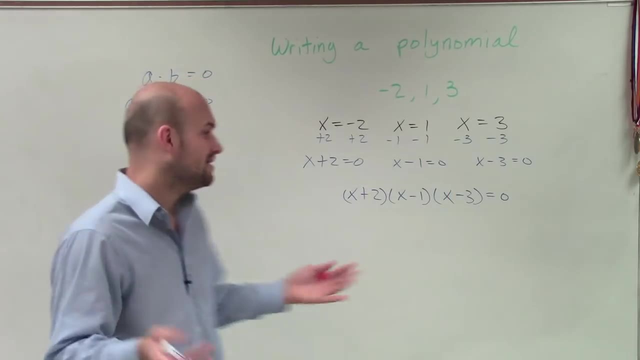 Because now we have a binomial times, a binomial times, a binomial, And the best way I like to approach this is just do one at a time. don't try to do everything crazy with this foil and moving stuff around. let's just do one at a time and the best way I like to do it. 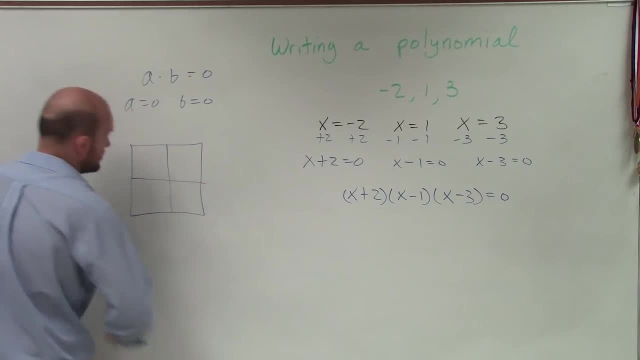 is just applying the box method to keep everything as organized as possible. so I'll just take, put one up here and then put the other binomial up top, then I just multiply through. so X times X is X squared negative X 2x negative 2. I can.